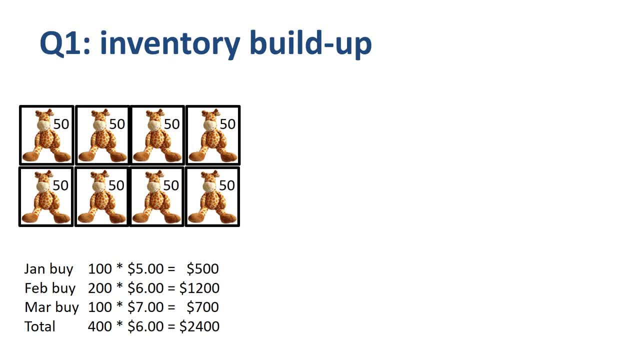 The company is 400 units and a total purchase price of $2400, so on average $6 per unit. In the warehouse the company does not specifically identify the boxes, they just stack them on a big pile For cost accounting and inventory valuation purposes. the company does keep track of the 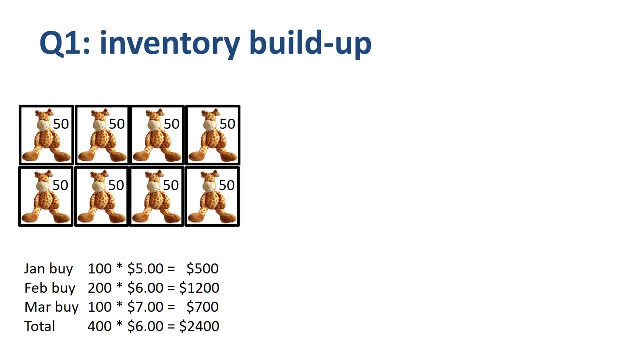 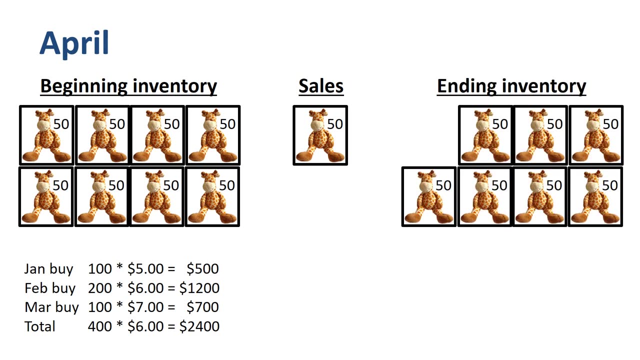 timing of the buys and the unit cost. Then we go to April. The ending inventory of Q1 is the beginning inventory of Q2.. The first box of toy giraffes, 50 units, is sold in April. The ending inventory is 7 boxes of 50 units each. 350 units in total. 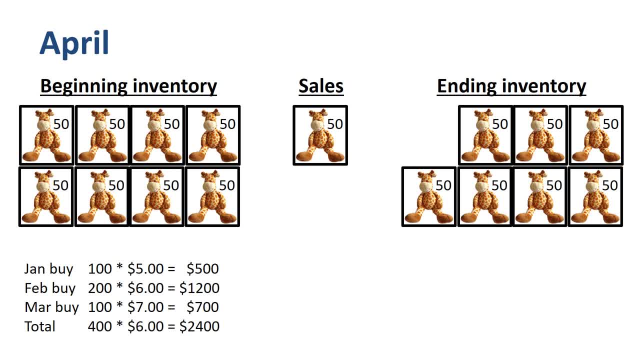 For inventory valuation as well as determining cost of goods sold, it is important to determine what is the cost per unit for this specific box. With FIFO first in, first out, we assume that the oldest inventory gets sold first, so we assume that the box sold. 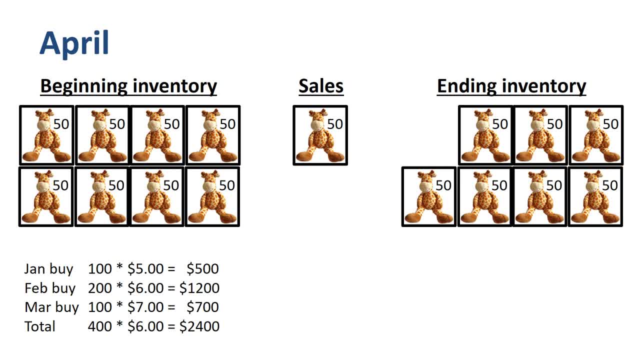 is originated from the January buy. What remains in inventory at the end of April is 50 units from the January buy, the full 200 units from the February buy and the full 100 units from the March buy. In total 350 units with a total purchase price of $2150, so on average $6.14 per unit. 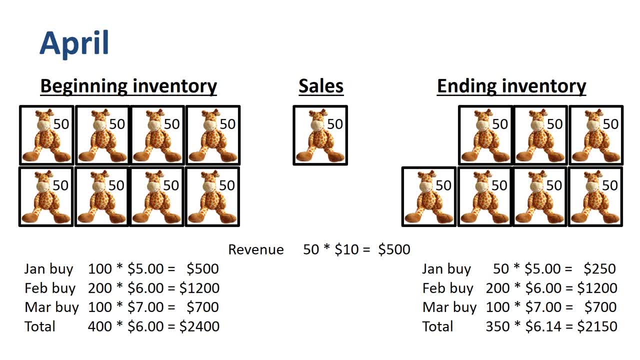 If we prepare the income statement for April, revenue is 50 units times $10.00, which is $500.00, cost of goods sold, or COGS, is 50 units times $5.00, which is $250.00, and 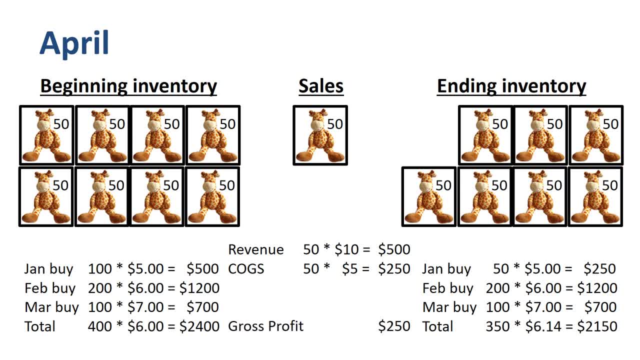 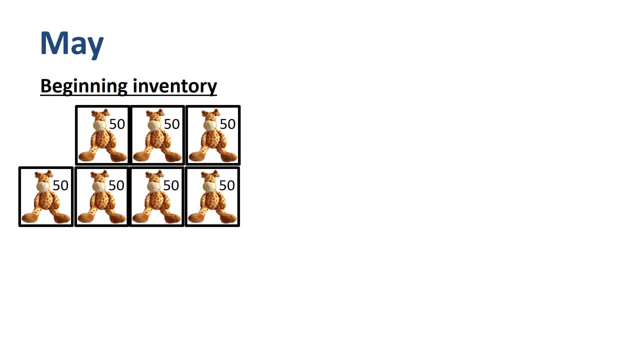 gross profit is $250.00.. Out of the January buy that was part of the beginning inventory, 50 units go to COGS and 50 units go to the ending inventory Onward to May. The ending inventory of April is the beginning inventory of May. 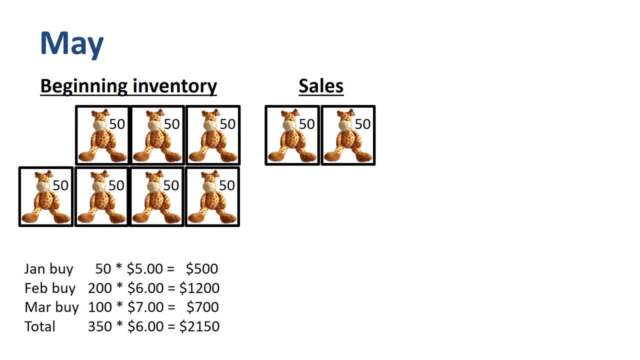 Two boxes of toy giraffes are sold in May. The first box of toy giraffes is sold in May. The second box of toy giraffes is sold in May. The ending inventory is five boxes of 50 units each. 250 units in total. 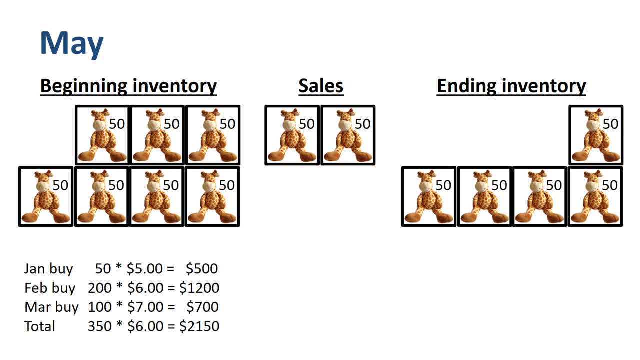 We once again apply FIFO first in, first out and assume that the oldest inventory gets sold first. What remains in inventory at the end of May is zero units from the January buy, 150 units from the February buy and the full 100 units from the March buy. 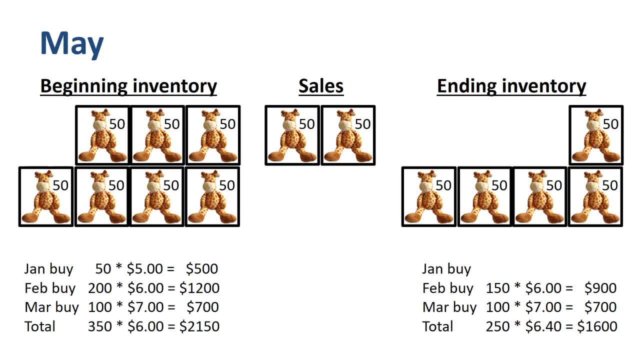 In total 250 units with a total purchase price of $1600. So on average $6.40 per units. If we prepare the income statement for May, revenue is: 100 units times $10 is $1000,. cost of goods sold, or COGS, is 50 units times $5 is $250, plus 50 units times $6 is $300,. 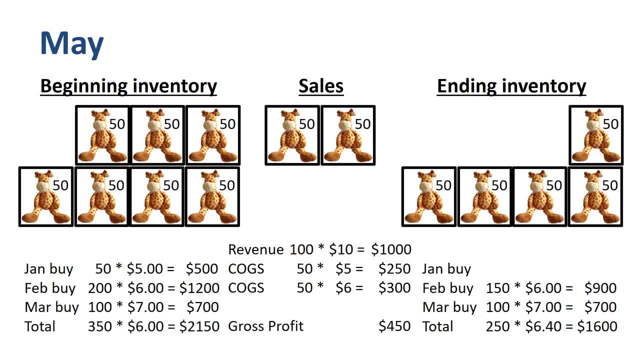 and gross profit is $450.. Out of the remaining January buy, that was part of the beginning inventory: 50 units from the beginning inventory. we took all 50 units to COGS and we took 50 units from the February buy into COGS. 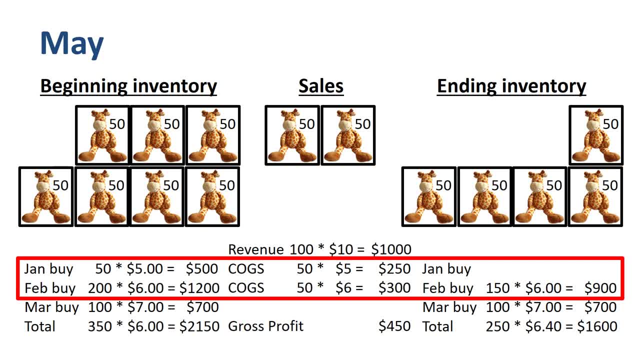 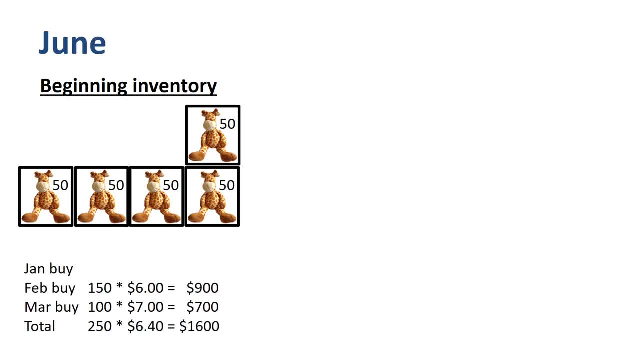 The remaining 150 units from the February buy go to the ending inventory Onward to June. The ending inventory of May is the beginning inventory of June. Four boxes of toy giraffes are sold. sales are really picking up pace. The ending inventory is just one box of 50 units each. 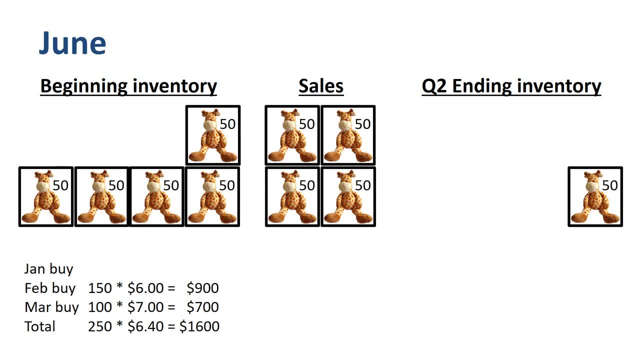 We once again apply FIFO First in, first out and assume that the oldest inventory gets sold first. What remains in inventory at the end of June is just 50 units from the March. buy 50 units of $7 each- $350 in total. 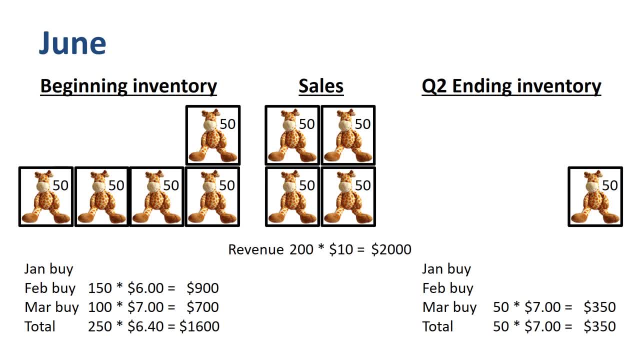 If we prepare the income statement for June, revenue is: 200 units times $10 is $2000,. cost of goods sold, or COGS, is 150 units times $6, is $900.. That's $2,000.. Plus 50 units times $7 is $350, so total COGS of $1,250, and therefore a gross profit. 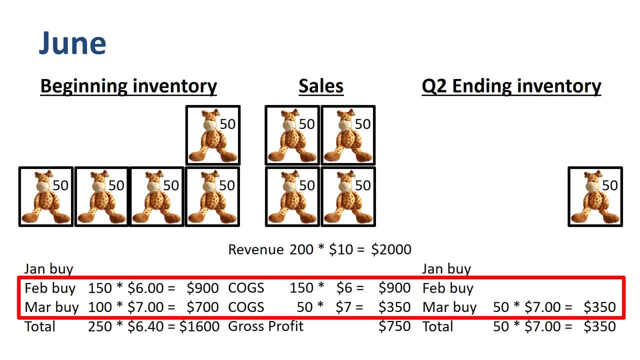 of $750. Out of the remaining February buy. that was part of the beginning inventory. we took all 150 units to COGS and we took 50 units from the March buy into COGS. The remaining 50 units from the March buy go to the ending inventory. 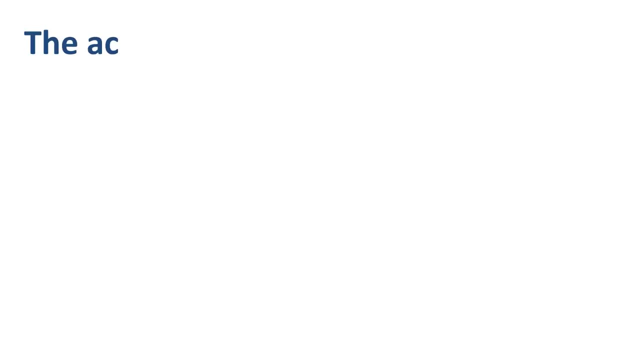 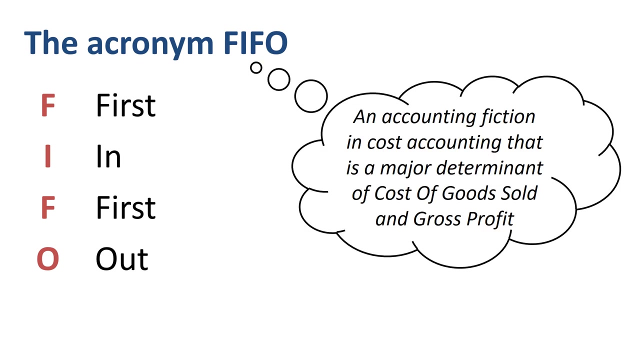 Summary and summary. Summary and summary. Summary and conclusion. FIFO, first in, first out, is an accounting fiction. in cost accounting that is a major determinant of cost of goods sold and gross profit. If cost per unit goes up over time and selling price stays flat, you make the highest profit.